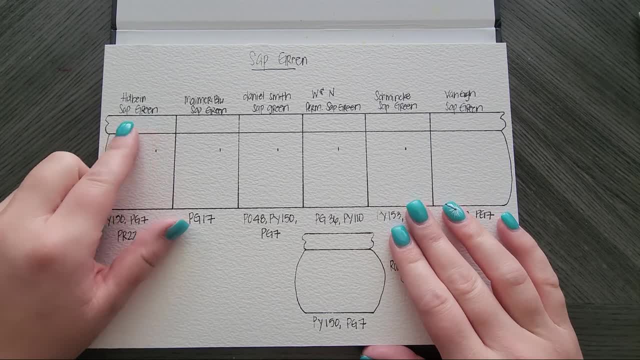 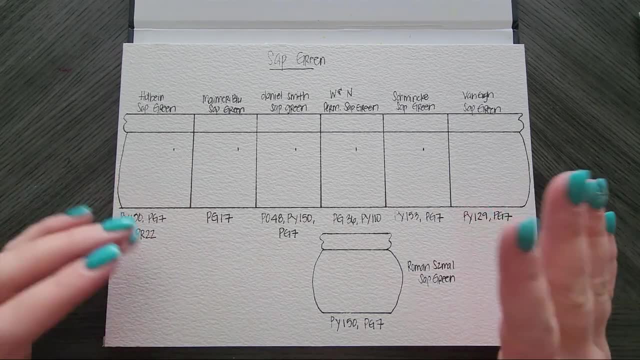 Schmal. So I'll be doing the mass tone and then getting it mixed with some water and dragging it down for you guys, just so you can see, and then we'll dry them up and then kind of talk about each one. So let's get started. 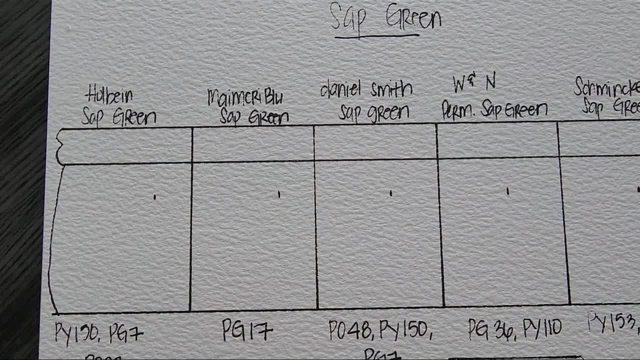 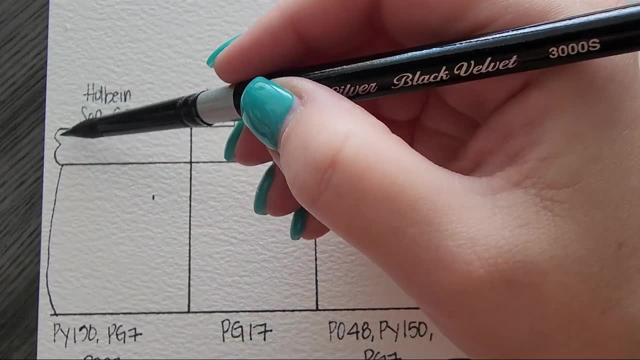 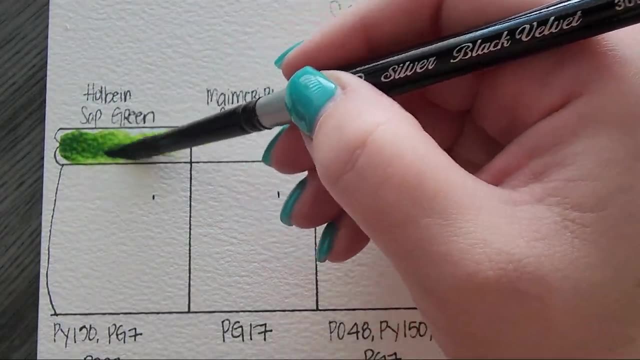 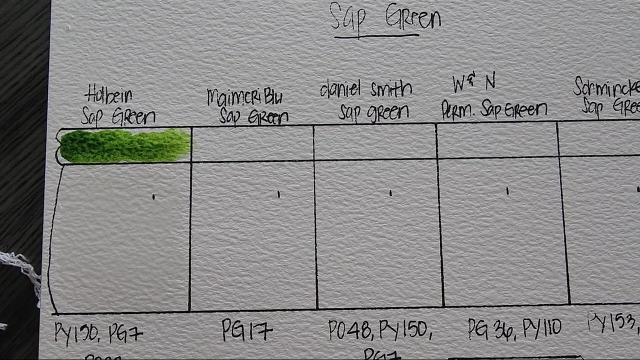 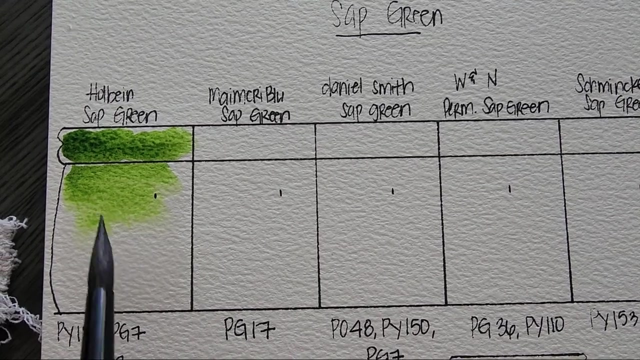 Okay, the first one we're going to start with is Holbein sap green. Now this is PY150, PG7 and PR22.. Some of these I am doing off of dot cards, some of these I am doing from tubes or pans that I 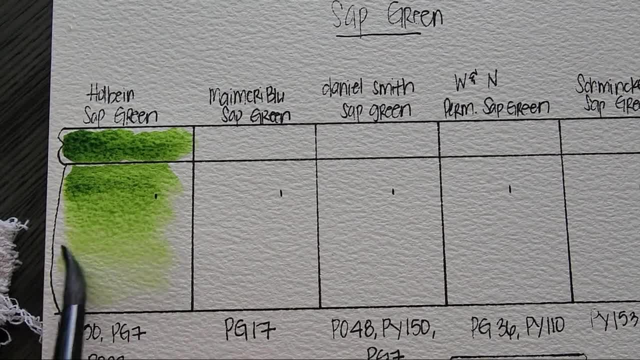 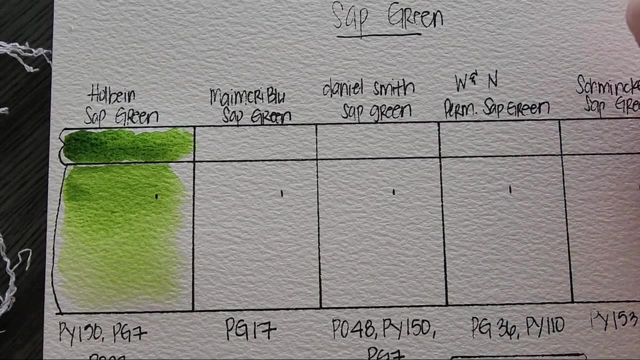 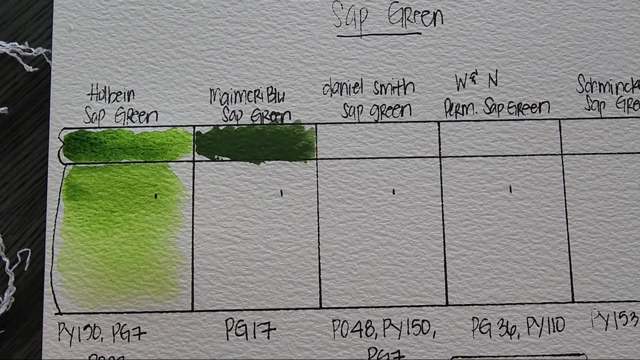 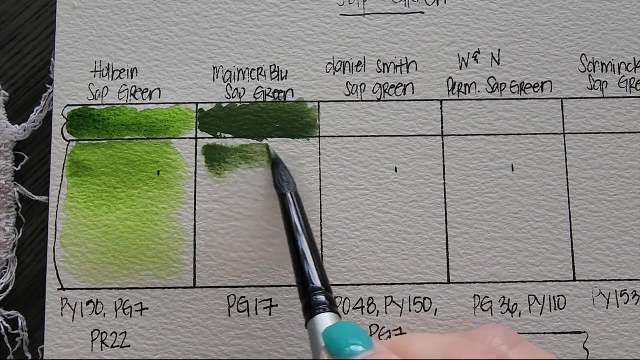 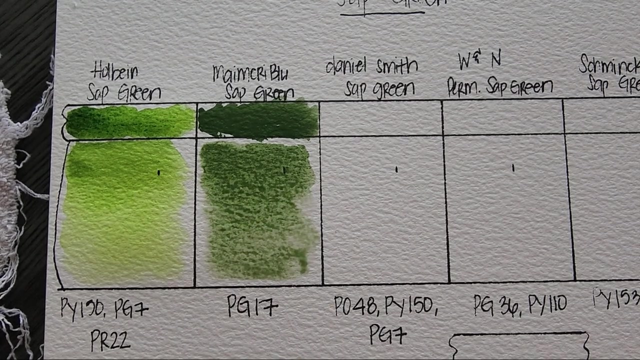 have for that color? it honestly just depends. Okay, next is my Mary Blue, sap green. This is the only single pigment color that you'll see, and that's PG-17.. I did just order dot cards for this one. That is quite the difference, but as 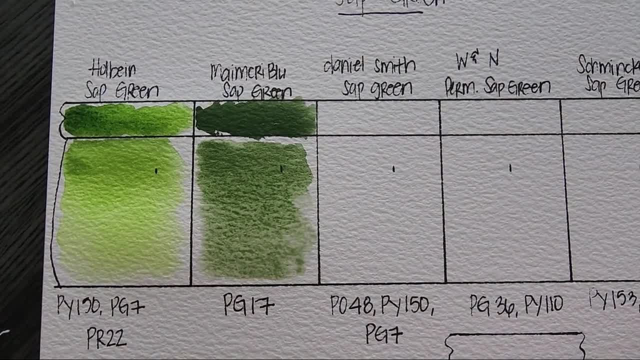 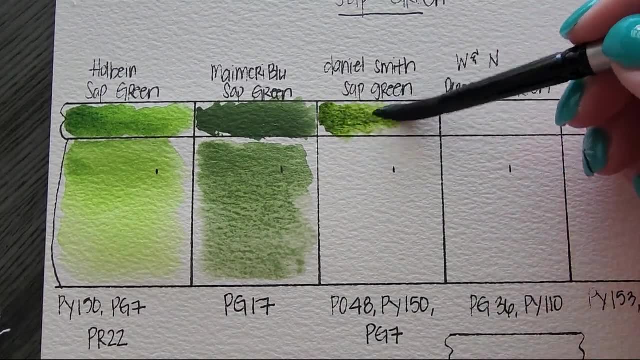 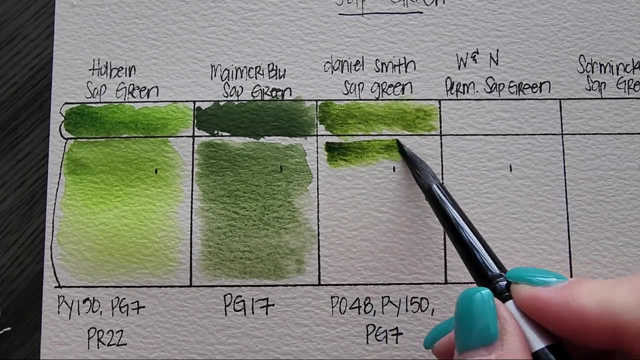 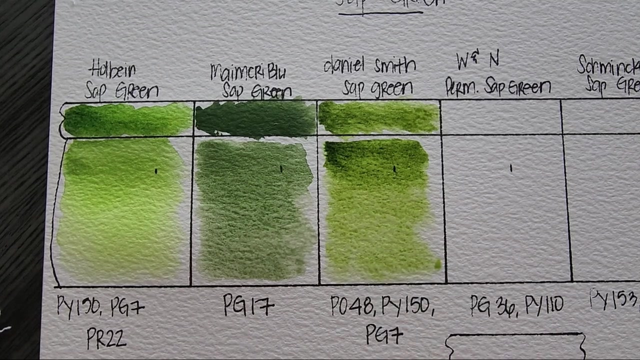 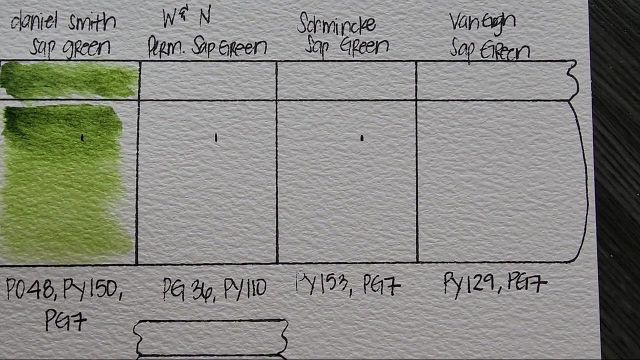 you can see totally different pigments. Okay, next up is the Daniel Smith Sap Green, which is PO-48,, PY-150, and PG-7.. Such a beautiful sap green, One of my favorites, I'm not going to lie. Okay, next we have the Winsor & Newton Professional, and this is called Permanent. 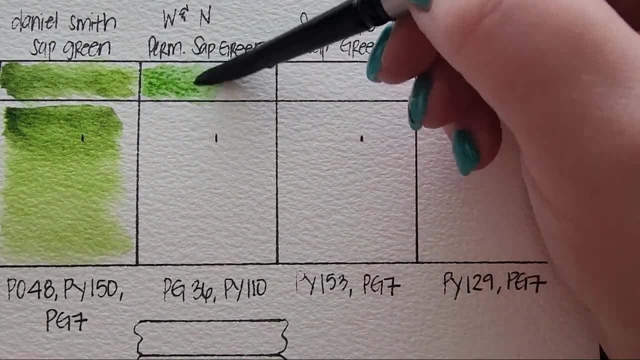 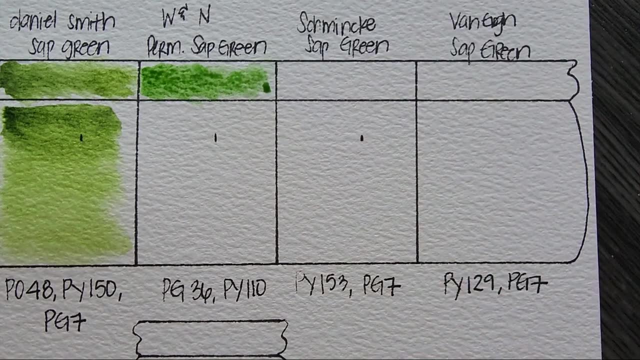 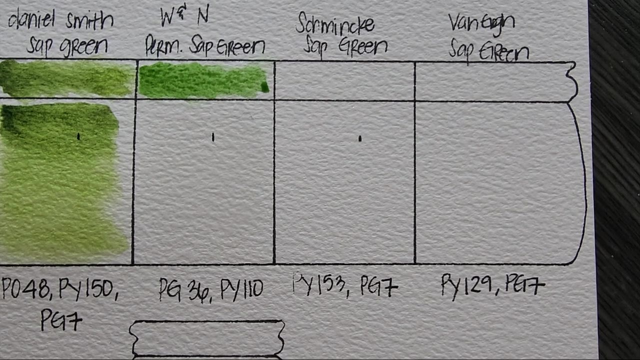 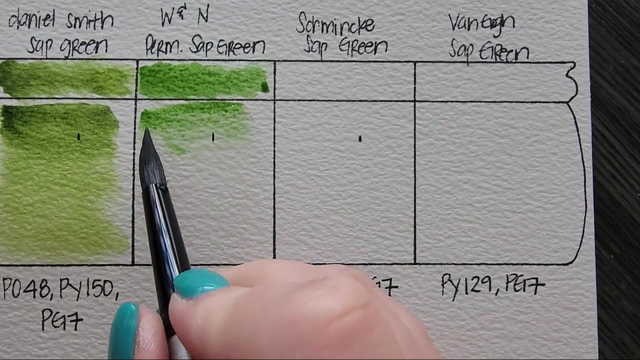 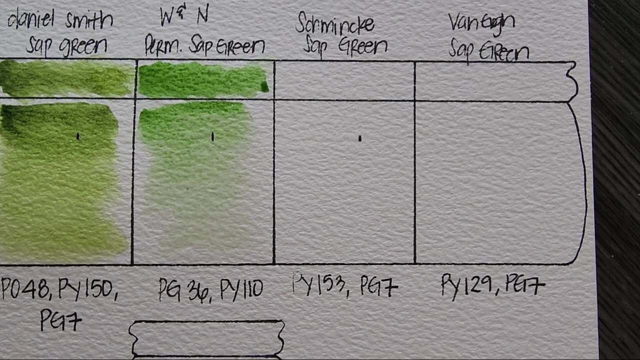 Sap Green, and it is PG-36 and PY-15.. I don't know if that one's going to give me enough pigment there. It's actually a pretty light sap green. Might not have a ton left on my dot card for that one. Okay, next is 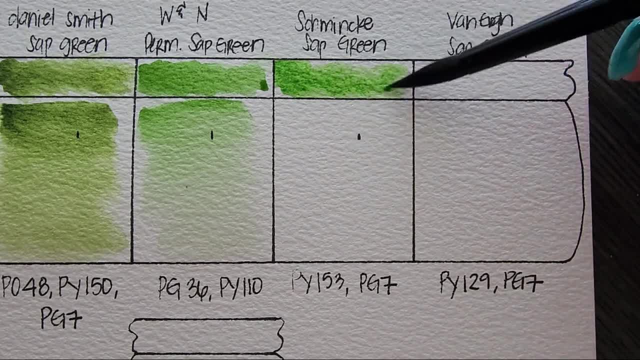 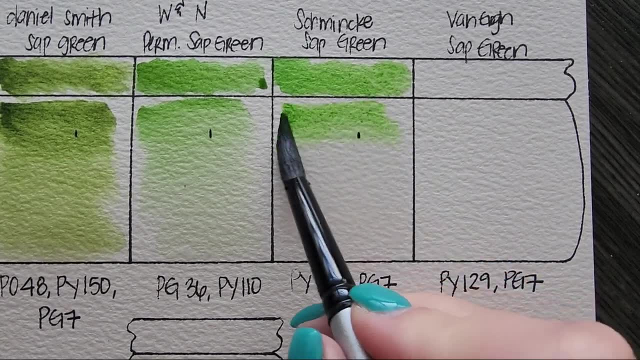 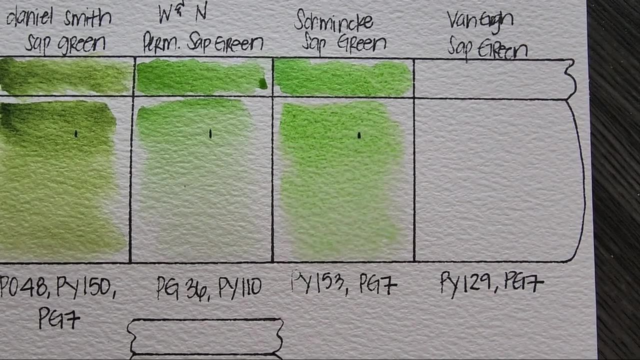 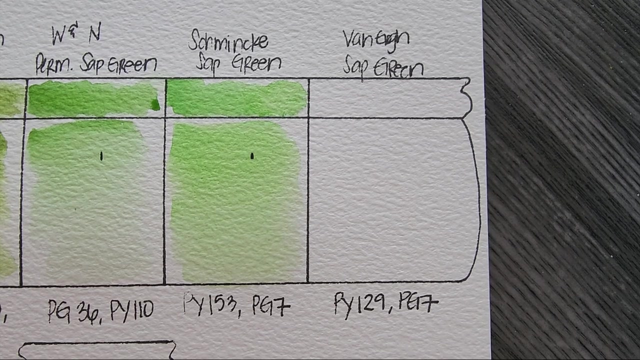 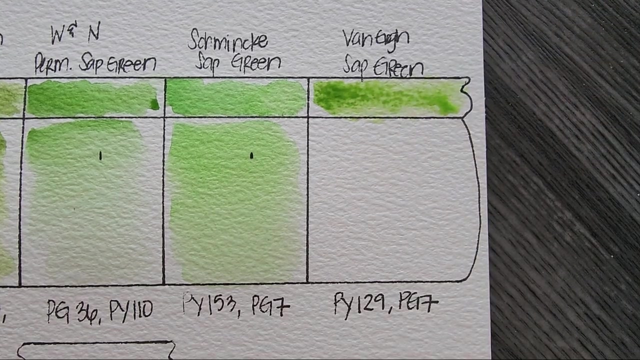 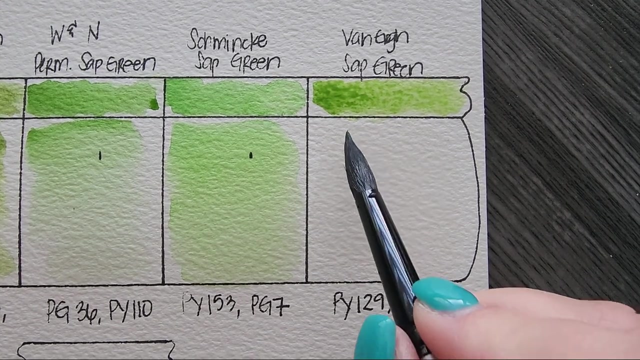 the Schmincke Sap Green, which is PY-153 and PG-7.. Very bright, Okay. off to the next. Okay. next is the Van Gogh Sap Green, which is PY-129 and PG-7.. I have to say Van Gogh and Daniel Smith give you a lot of paint in their dot cards, whereas 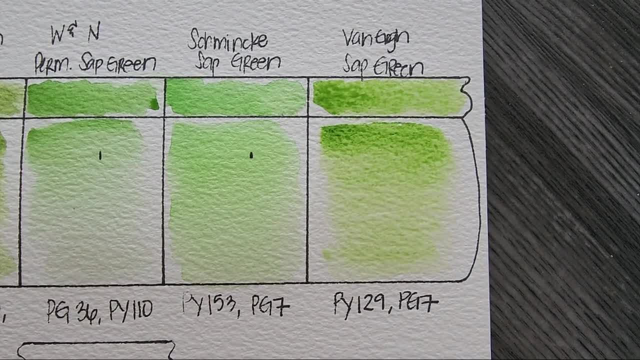 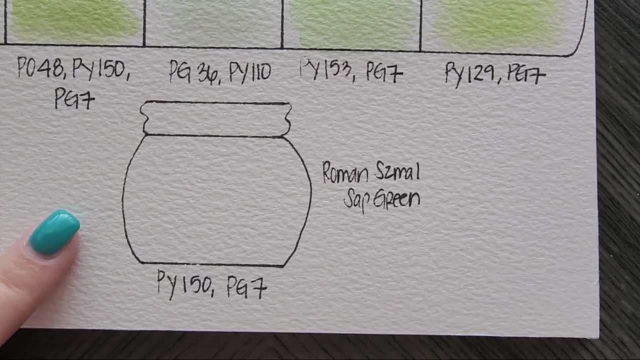 it kind of feels like Schmincke and a few others are lacking. Okay, now we are on to Roman Schmall Sap Green, which is PY-150 and PG-7.. Okay, now we are on to Roman Schmall Sap Green, which is PY-150 and PG-7.. 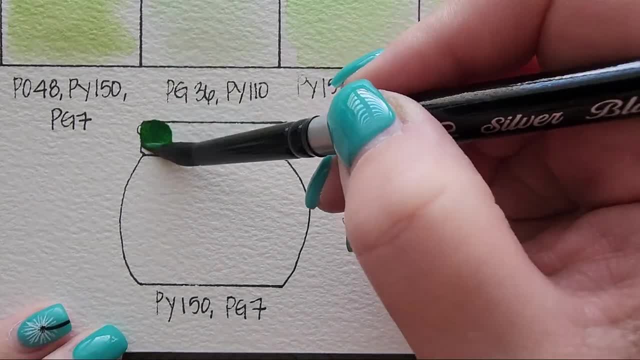 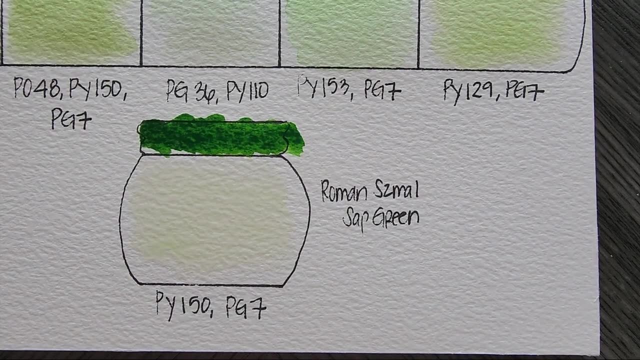 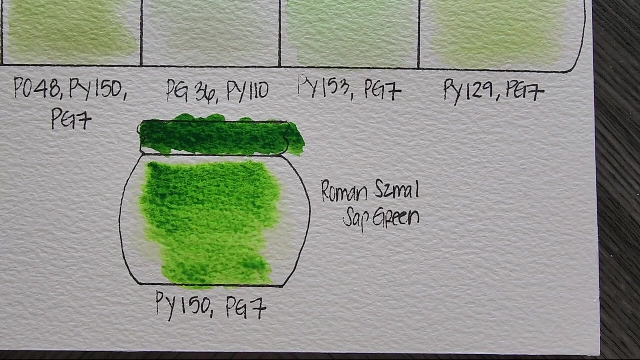 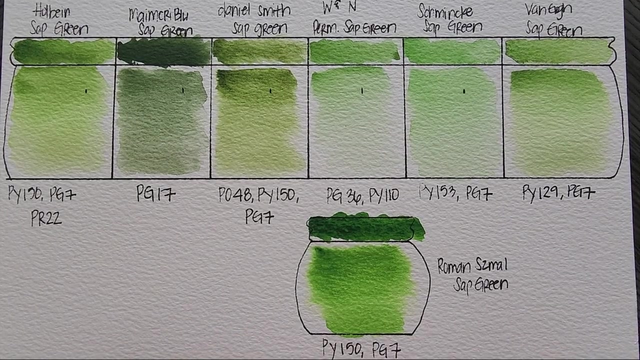 Okay, now we are on to Roman Schmall Sap Green, which is PY-150 and PG-7.. And it is a very dark one. This is actually in my Roman Schmall palette. Okay, let's have those dry up and then we'll come back. Okay, so this is exactly why I always say: don't. 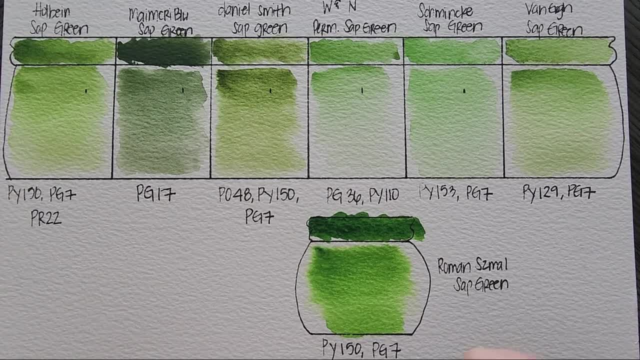 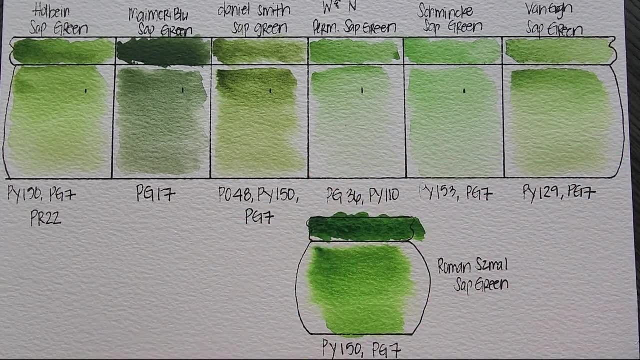 pay attention to the color name specifically and really get to know your palette and also your pigments. sap green is one of my favorite examples and as you can see why. so, first of all, you can see that most of these have a different range- quite a few. 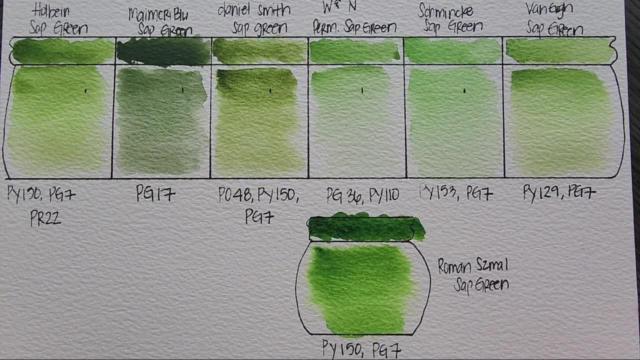 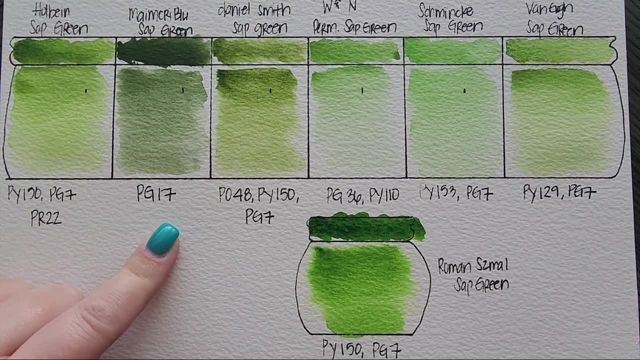 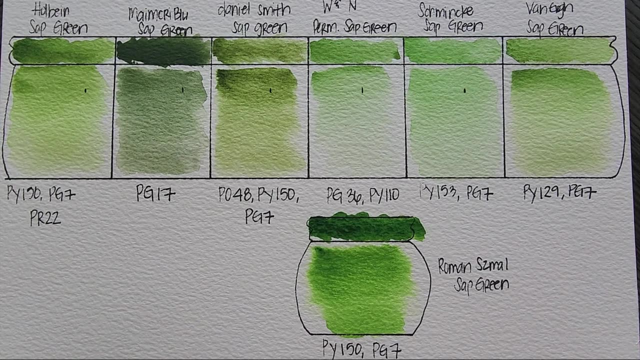 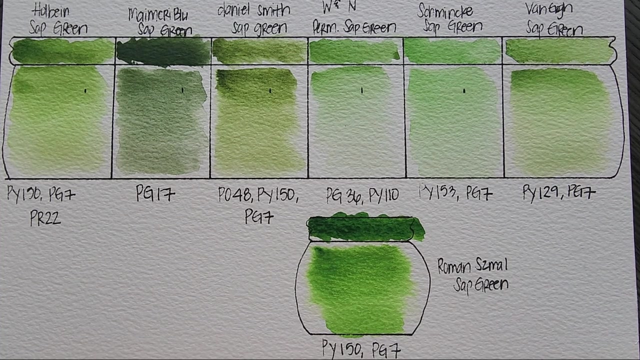 do use PG 7, but PG 17, only my Mary blue is the only one that has that pigment. I believe the same goes for the PY 129. you know everyone makes their own mixes and their own idea of what a sap green is. but also look at the range in terms of. 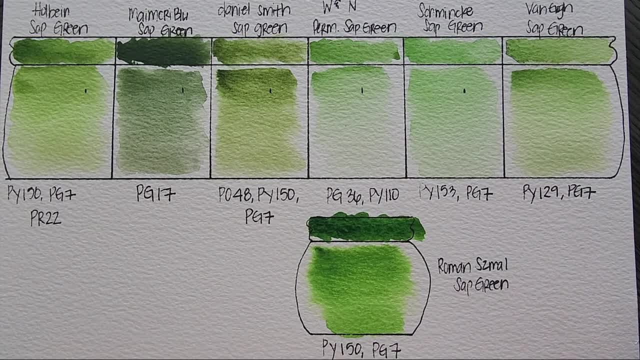 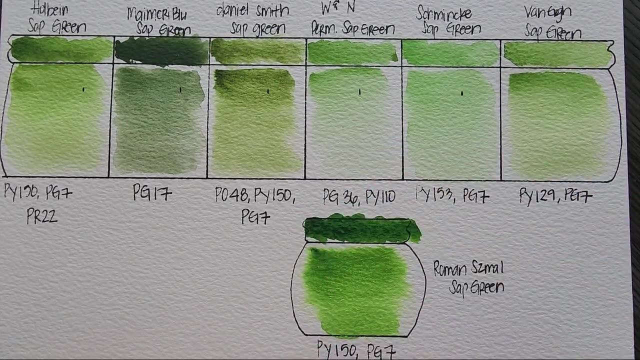 darkness and lightness and even earthiness. to be quite honest, the Daniel Smith one has a little bit more of that olivey color to it. the Roman small is dark when you do it mass tone or wet-on-dry, which is typically how I paint. so that's the color I'm going to. 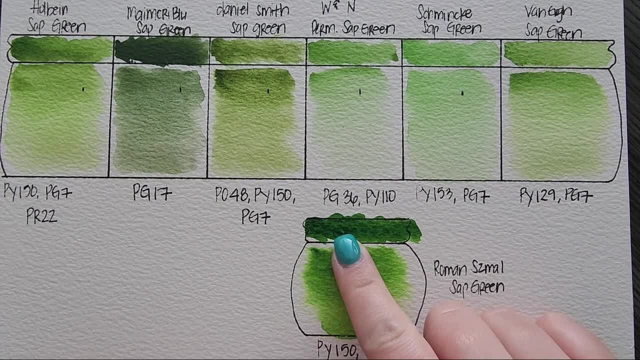 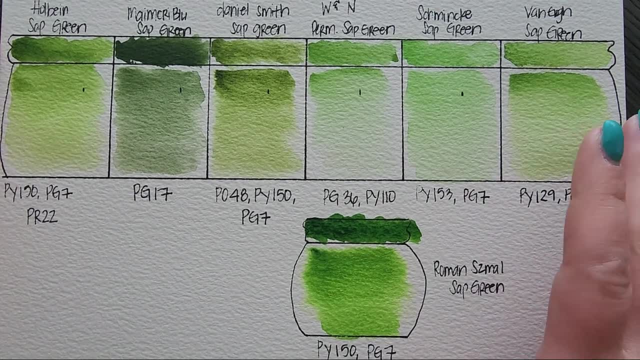 get unless I water it down on my palette. let's see how dark that one is like, how dark the my Mary blue is as well. Holbein sap green is actually quite pretty, prettier than I remember it, the Windsor and Newton sap green. I'm not a. 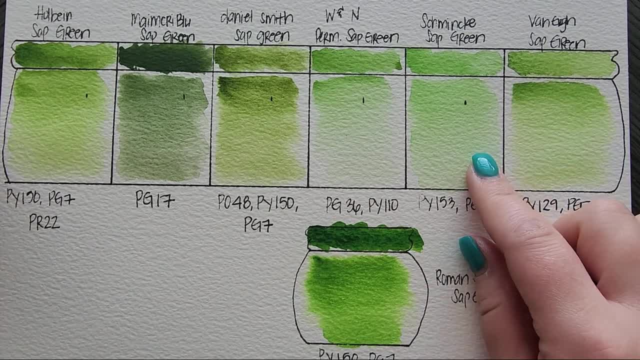 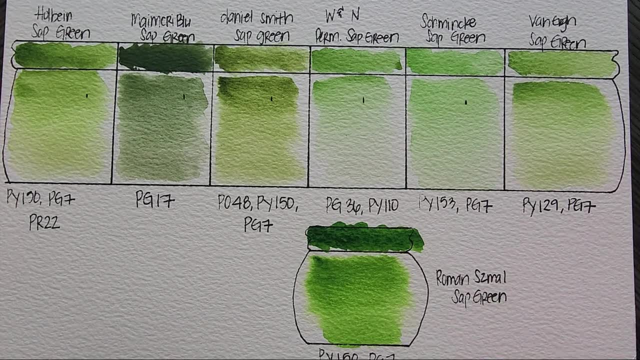 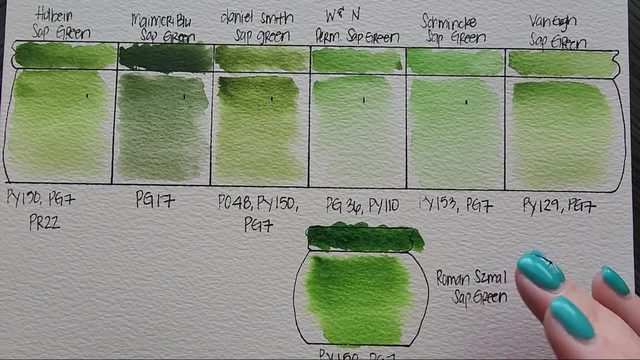 big fan of- I'm not gonna lie to you- and same with the schmincke. it's just so bright. and then the Van Gogh sap green is actually not too bad. but if I had to pick favorites, obviously I enjoy the Roman small sap green. it is in my Roman. 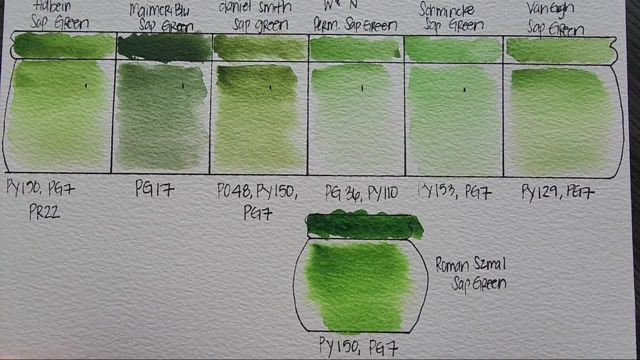 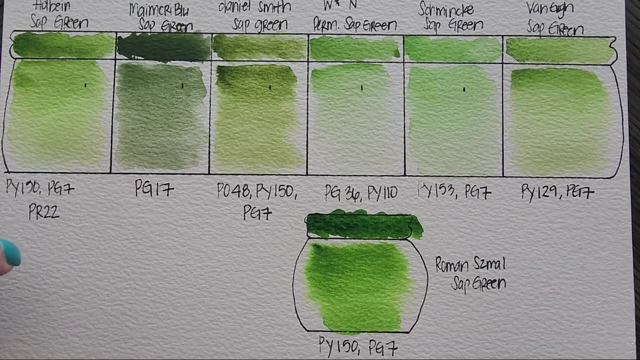 small palette. so, that said, I honestly think my favorite sap green might even be the Holbein. I love the color. it's bright because this one, the Daniel Smith one, does have that kind of all of the undertones, but it's a little bit more down and I just don't picture that with the sap green. so this one's bright, but 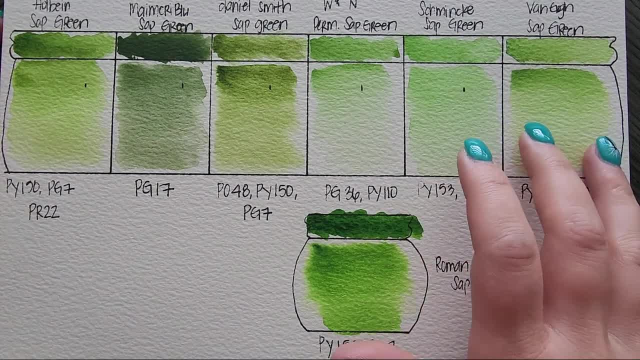 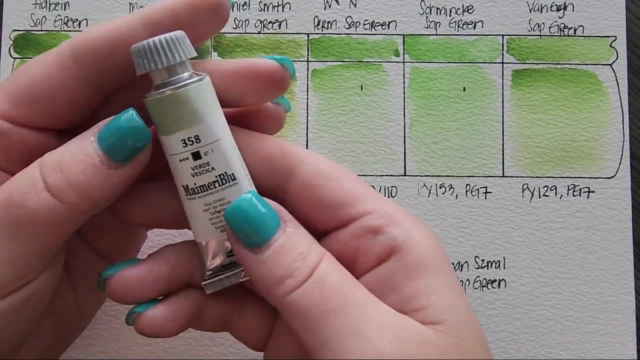 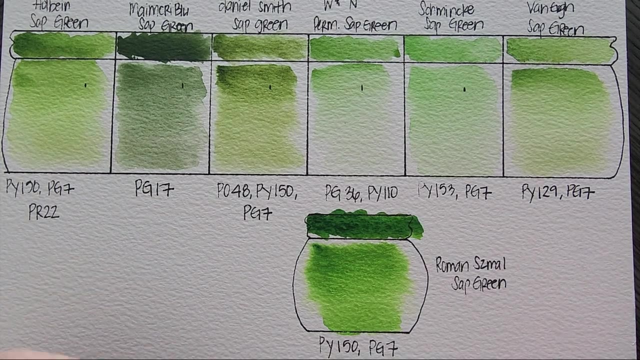 it's not super bright like the schmincke. that said, the my Mary blue one is quite pretty as well, so I ended up actually buying a tube of that one, by the way, and it does kind of remind me of a terra verde color, but it says sap green on it. 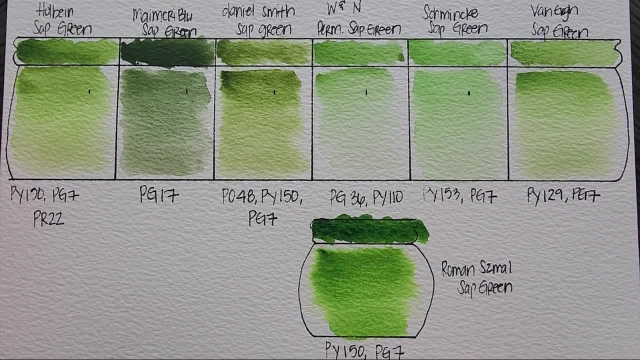 but again that's why I don't pay attention to it, because I don't want to too much to names and I'm particular. I look at the pigments pg7, like I said, normally when I see that I'm not surprised. but yeah, I mean I'd have to. 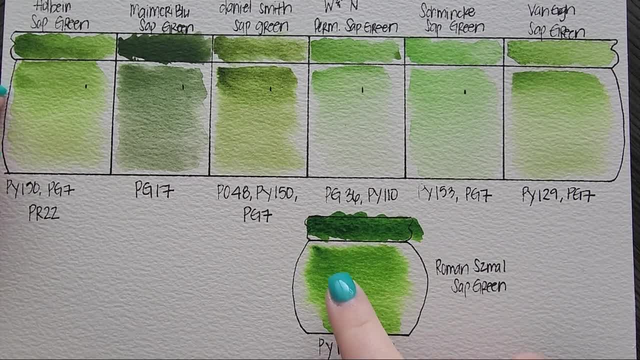 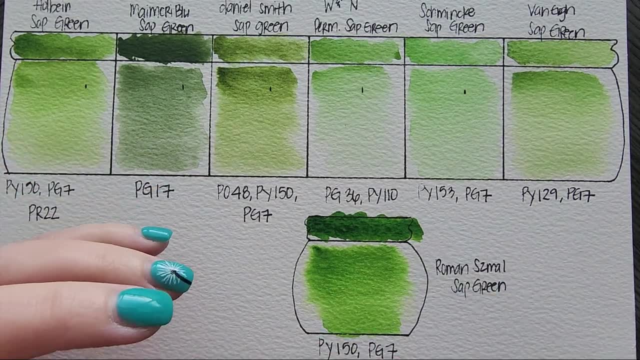 say I'm really liking the Holbein. of course I do like the Roman small Daniel Smith is in there just because it's earthy. however, I wouldn't really use it in. my palette is one of my brighter greens and then my Mary blue is actually.